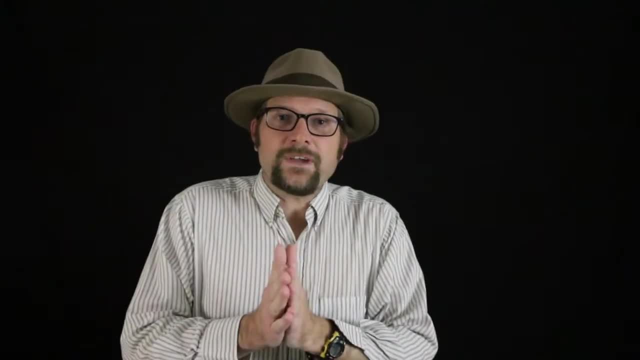 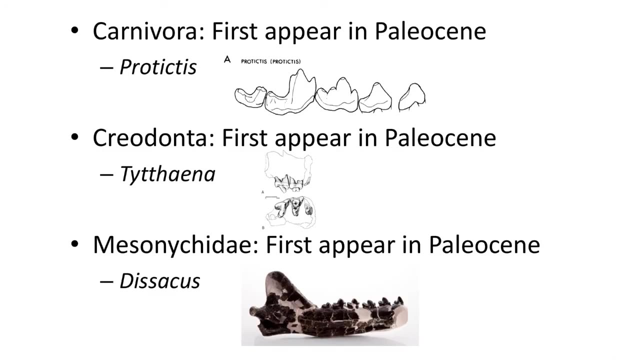 teeth late in their evolution. All right, so let's look at the earliest members of the ecosystem, members of each of these three groups In the Paleocene, the first three carnivorous mammals living in the new air after the extinction of the dinosaurs. Among the carnivora, we 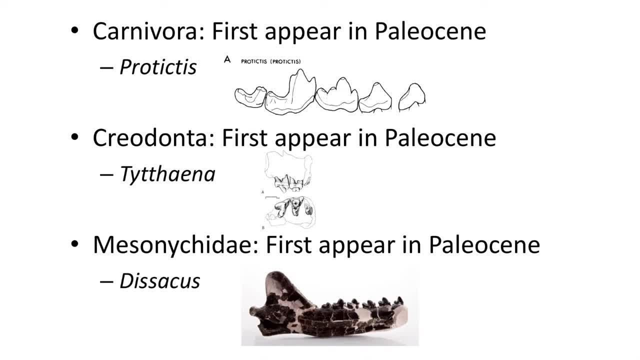 have Protictus, which has a large lower first molar as the sole carnassial tooth, With Creadanta. we have Tahiana, which has multiple carnassial teeth With Mesonicidae. we have Didysicus. 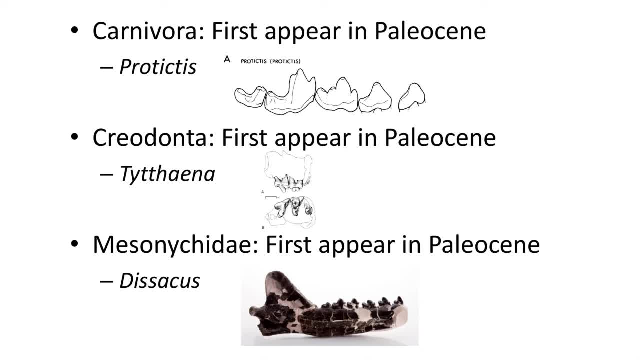 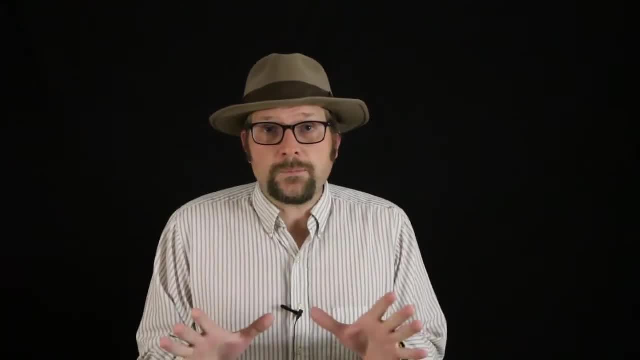 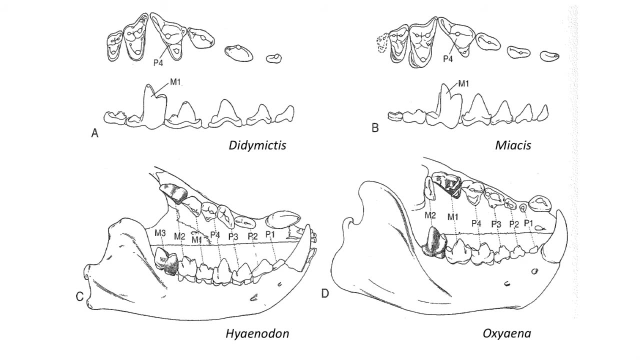 with a row of multiple sharp teeth that are somewhat carnassial in nature but are more simple, kind of scissor like teeth. Now, all of these Paleocene carnivores are about coyote or smaller size By the Eocene here in North America. 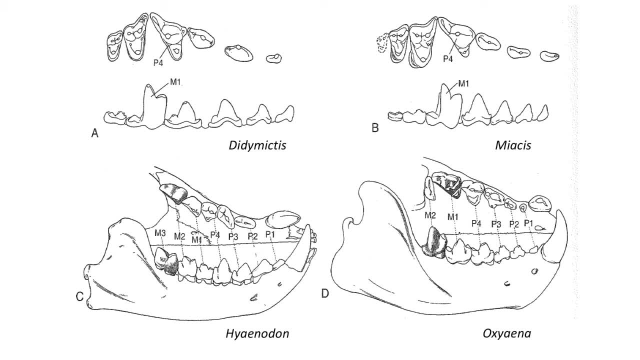 carnivorous mammals got larger, to be about the size of a wolf. The top two carnivores display carnassial teeth that involve the upper fourth premolar and the lower first molar. This is what is found in cats and dogs today, and Diomedicus and Miasis are more. 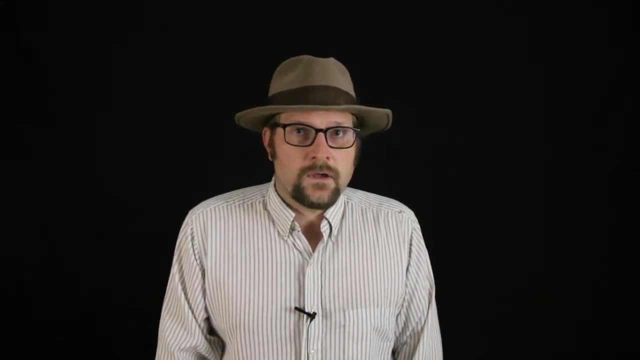 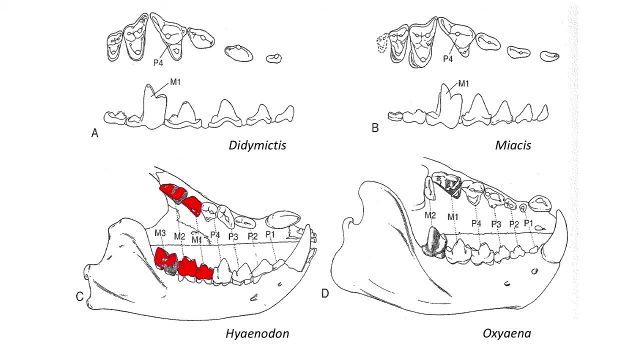 closely related to cats and dogs. The lower figured Eocene mammals are Hyenodon, in which the upper, second, third and fourth premolar, as well as the entire lower molars, are all carnassial teeth. This defines a group of Creadant mammals. 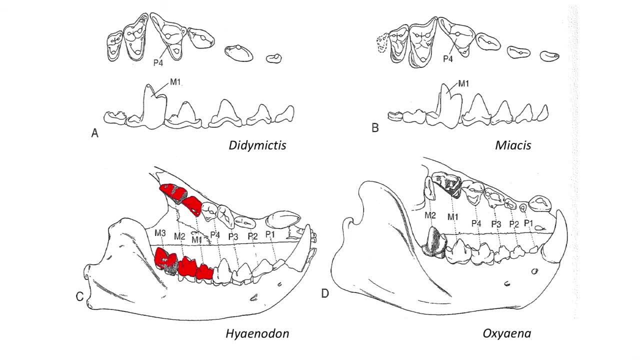 called Hyenodon today, while the Eocene mammals on the lower right in the figure is Oxyhena, which is also a Creadant, but exhibits a carnassial occlusion between the upper first premolar and the lower third premolar. The lower third premolar is called Oxyhena, which is also a. 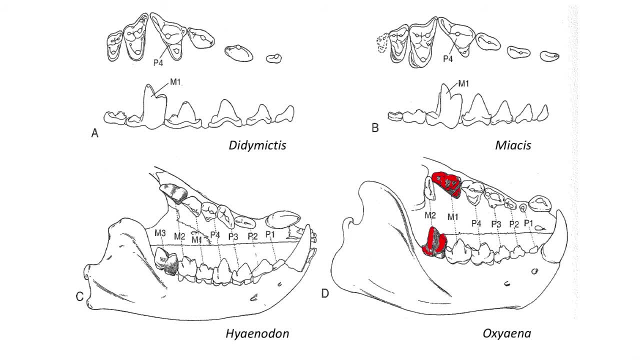 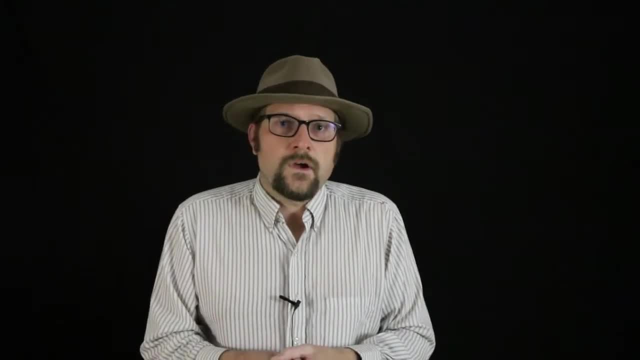 Creadant, but exhibits a carnassial occlusion between the upper first premolar and the lower third premolar. This mammal is an Oxyhenid Creadant. The Oxyhenidae Creadants were large lion sized mammals that lived during the early Eocene. 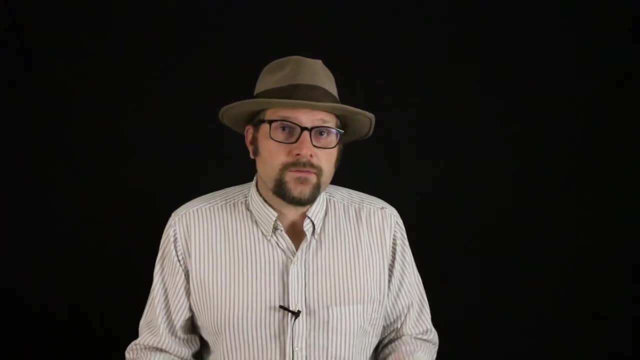 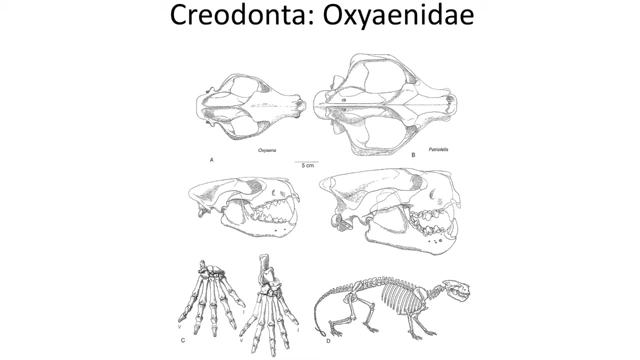 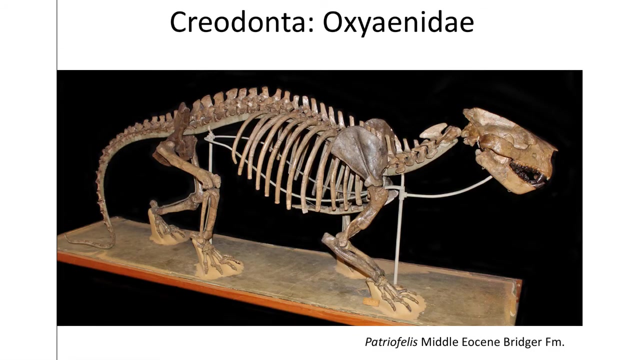 and which are well known in the American west but are also found in Asia and Europe. They had very short skulls that somewhat resemble the skulls of modern big cats. Some of the The coolest oxyhenid is Patrophelus, which is known from the Middle Eocene Bridger Formation. 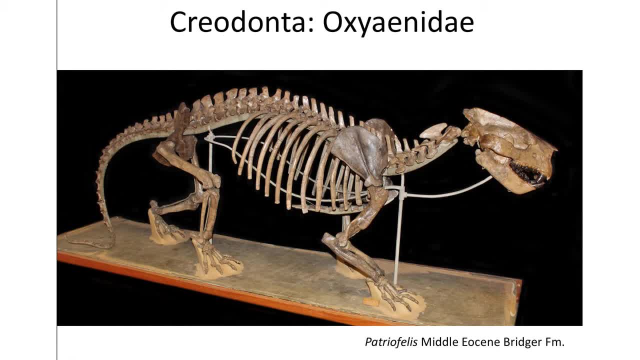 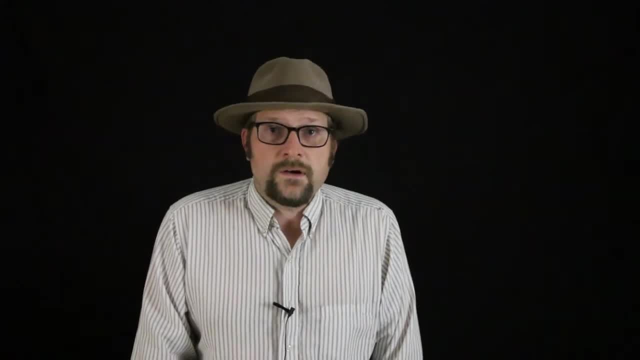 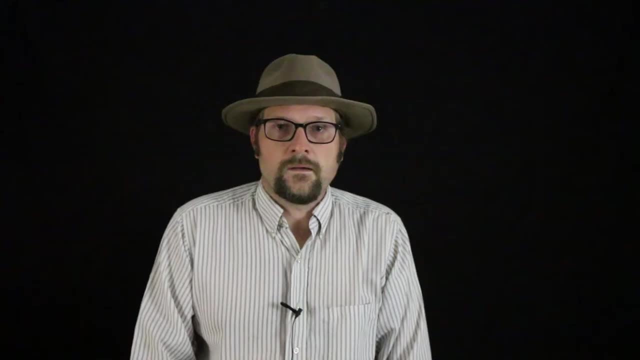 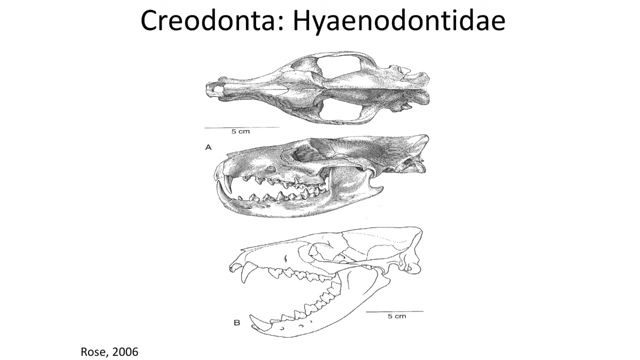 of southwestern Wyoming. It's known from some nearly complete skeletons Living also during the early Eocene were the smaller Hyenodontidae which, unlike the oxyhenids, had multiple carnassial teeth. The hyenodontids had longer skulls and were weasel to small dog sized mammals, some with 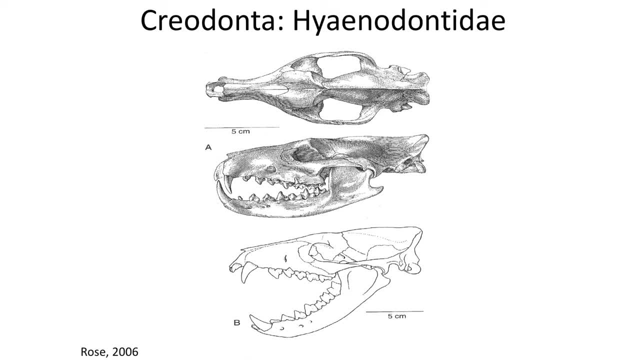 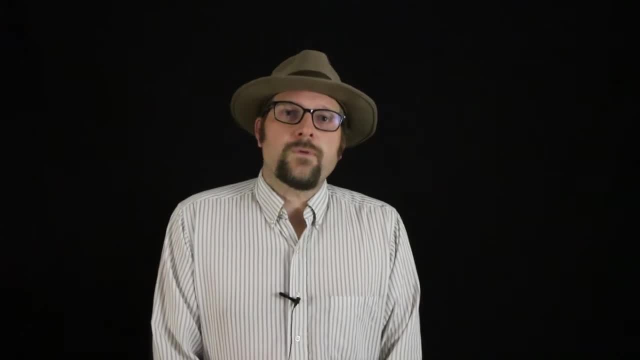 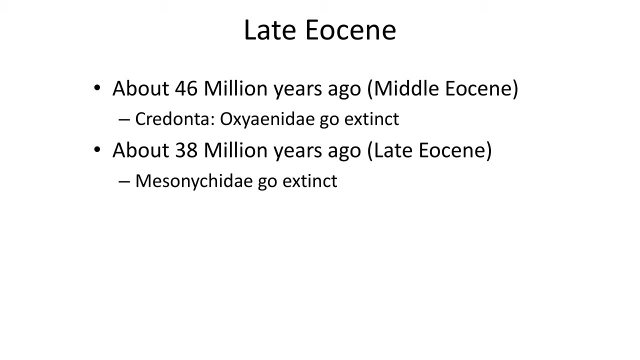 the ability to climb trees. Some of the larger ones during the Middle Eocene include Cynopa and Prolymda scion. Then, around 46 million years ago, the larger lion sized oxyhenids went extinct and by around 38 million years ago, the bear sized mesonychids went extinct. 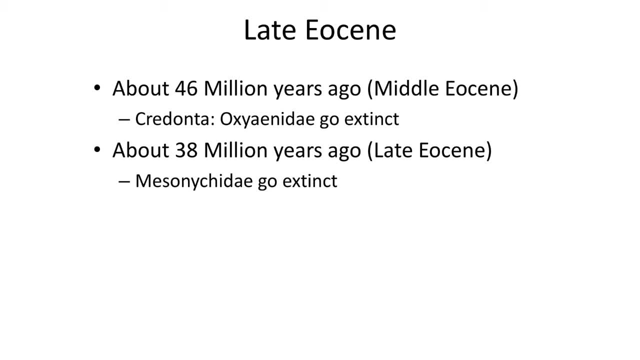 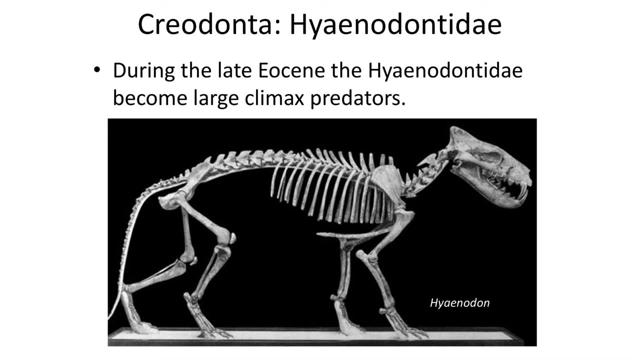 Which meant that during the last few million years of the Eocene, large mammal carnivores were replaced by the hyenodontids, which went from weasel sized mammals to large wolf sized mammals like the late Eocene Hyenodontidae, creodont hyenodon. 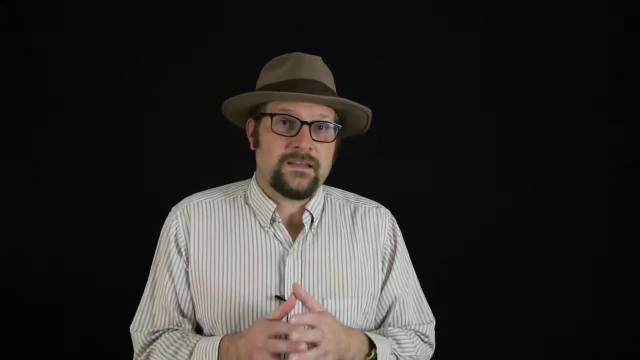 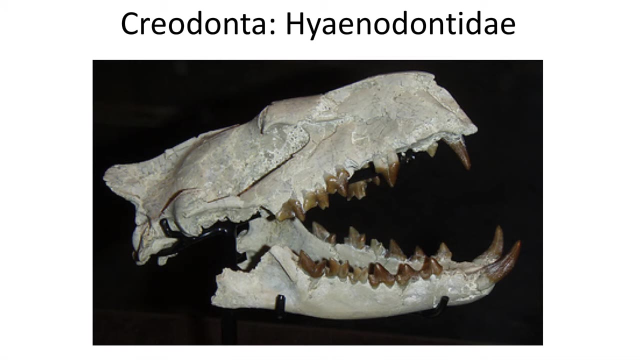 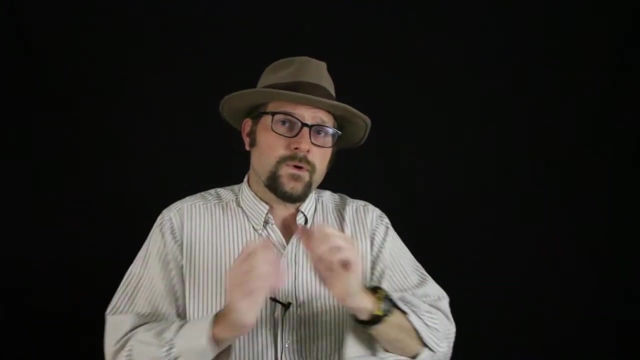 Hyenodon was the climax predator during the late Eocene and also represents one of the last of the hyenodontids to exist before their extinction at the end of the Eocene. The Eocene-Oligocene boundary was important because, while many carnivores lived through, 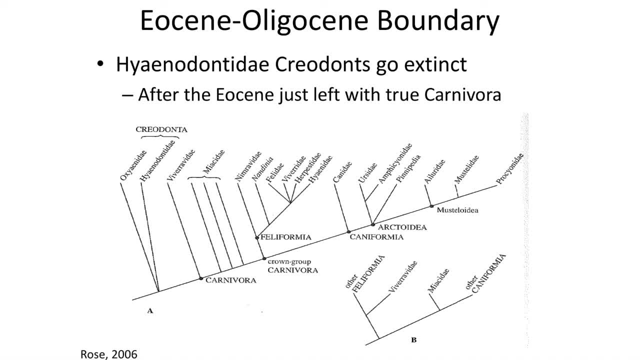 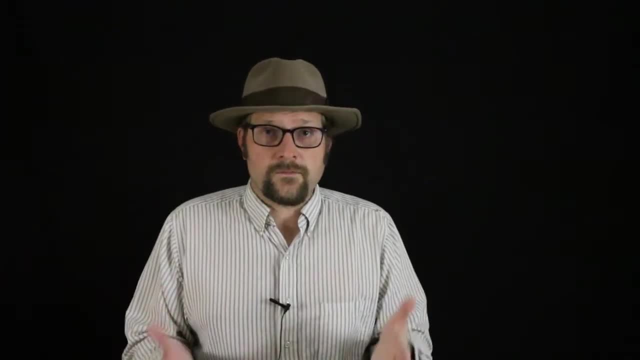 this event, the creodonts finally succumbed to extinction. The carnivora survived. these survivors would evolve into cats, dogs, bears, weasels, pinnipeds and hyenas. Among the Eocene, carnivora were a group called the myasidae, which closely resembled small 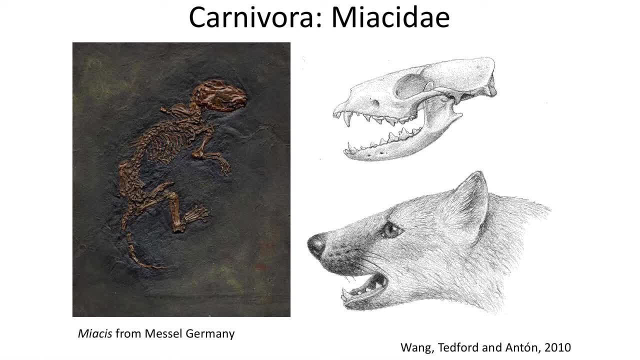 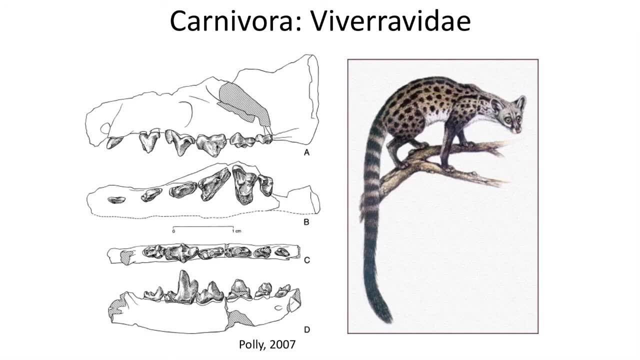 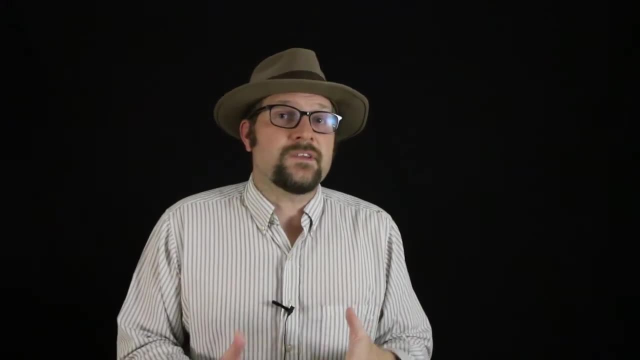 dogs or coyotes, some of which were arboreal while others were more terrestrial. The other group of Eocene carnivora were the vivaravidae, which were civet like mammals For many years. the vivaravidae were placed in the filiforma. this is a large branch that 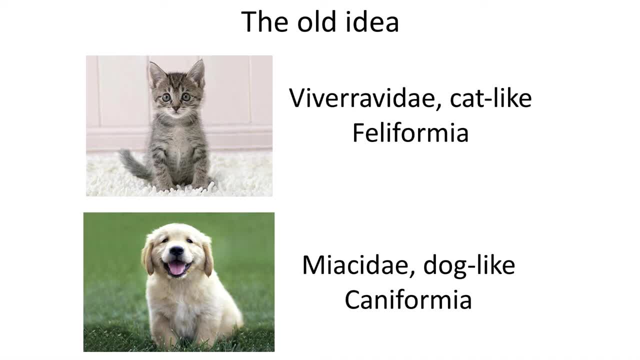 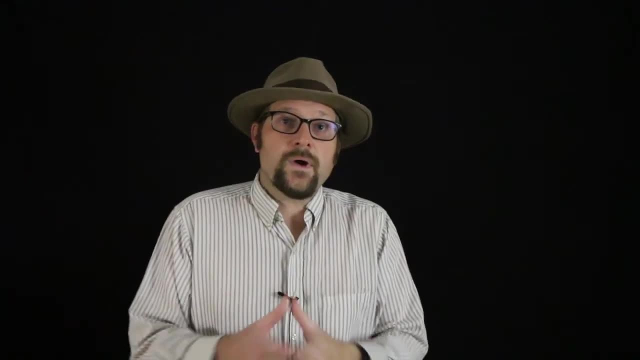 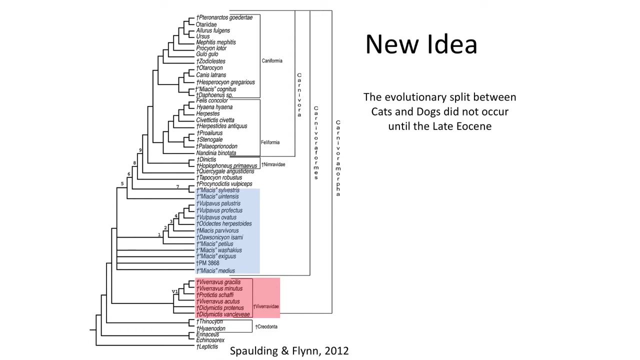 would lead to cats, while the myasidae were placed into the cainiforma as ancestors to dogs. thus, the dog-cat split in evolution occurred early within the group. However, more recent work has argued that the vivaravidae and myasidae are early splits. 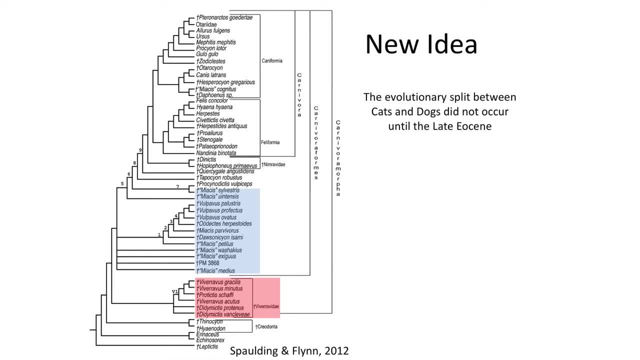 off the tree and are not ancestral to either cat. They are not even grouped within carnivora. they are grouped in a larger grouping called the carnivora morphs. Some of the myasidae are closely related to carnivora, like Tapa scion, the Middle Eocene. 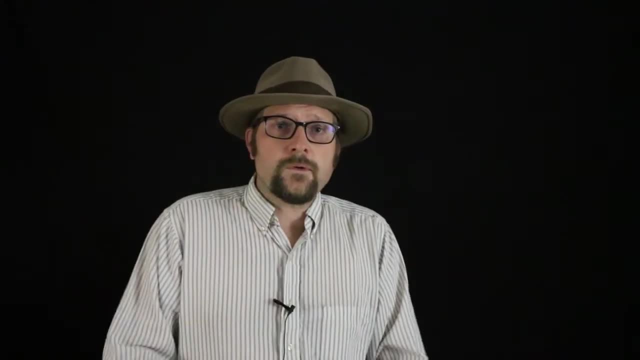 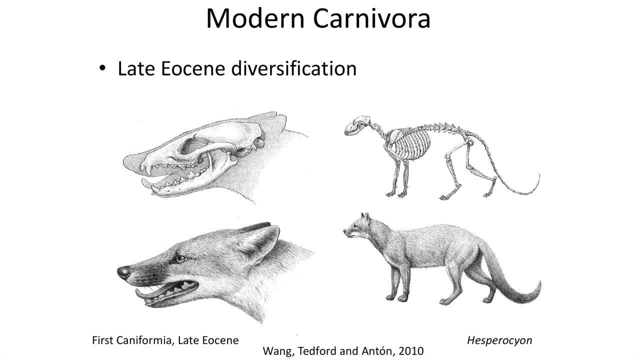 carnivorous mammal known from Utah. In this new scheme, the first true carnivora are the early cainiforma Hesperocyon. Hesperocyon is from the Lysidae Late Eocene of Colorado, which was a fox-like carnivore. 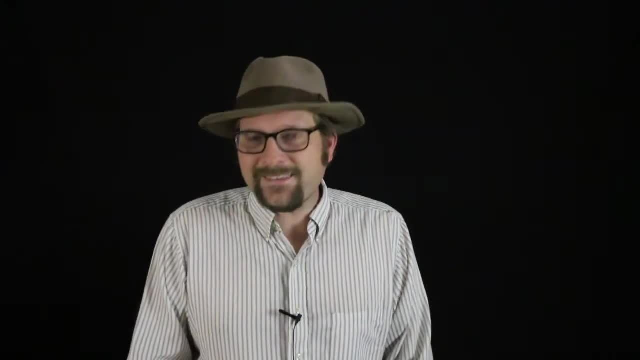 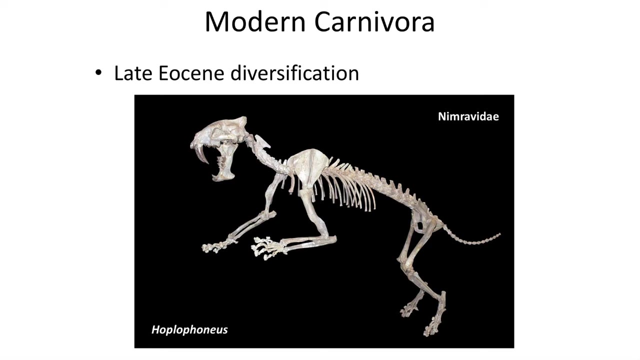 Now there is one other group that shows up at the end of the Eocene called the Nymravidae, which are known also as the false saber-toothed cats. They have many cat-like features, like retractable claws and saber-like teeth, and the most well. 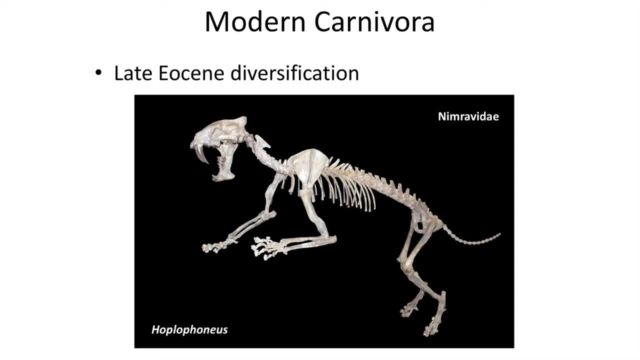 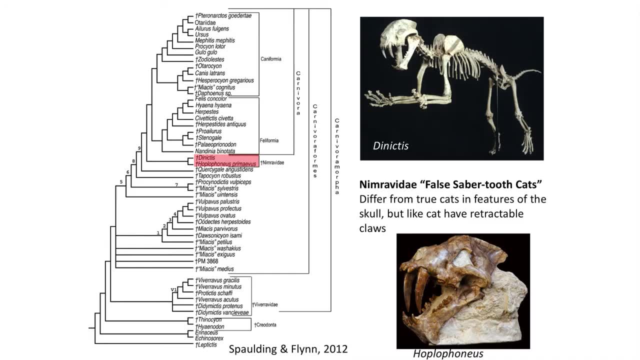 known is Hopiophonus from the White River Formation of Colorado. These early saber-toothed cats lived at the end of the Eocene and are the sister group to the crown branch of Carnivora. We will see the evolution of saber teeth twice as later on within the cat family. they will 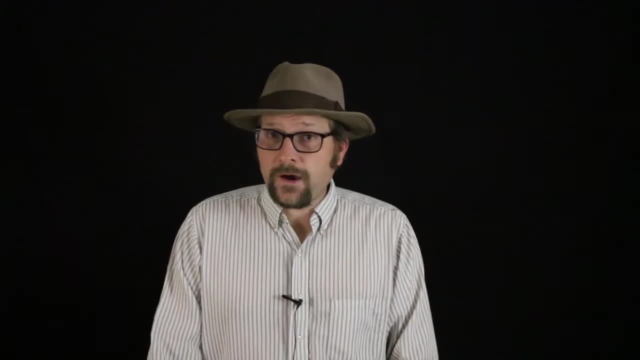 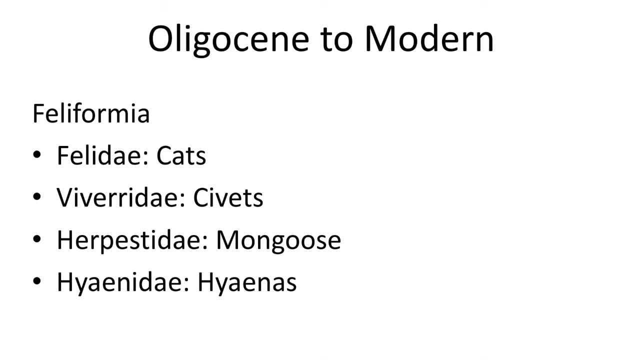 appear again From the Oligocene to modern epochs, two groups would remain. the first group, the Filiforma, includes four families: the Filidae, the Viridae, the Sivits, the Herpestidae. 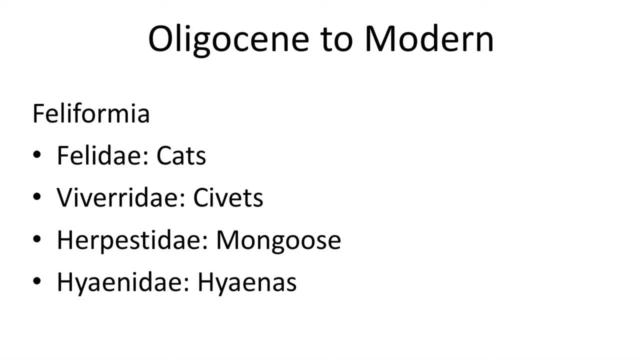 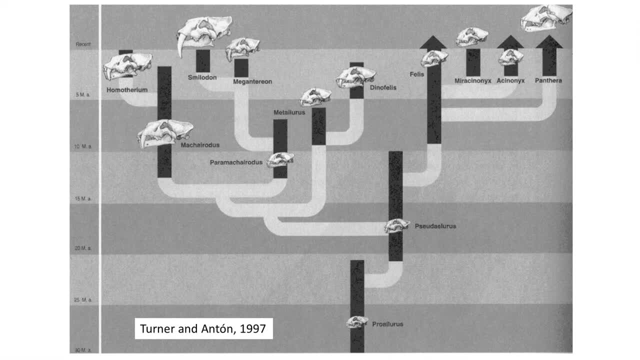 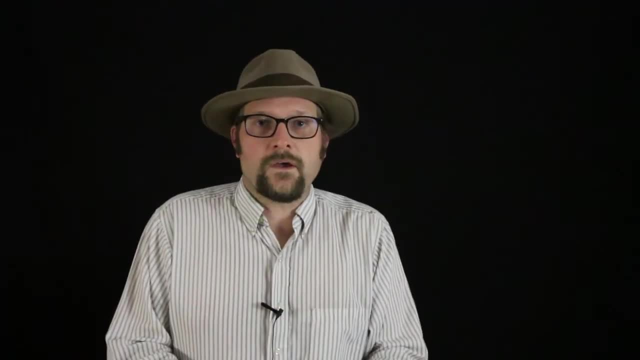 the Mongooses and the Hyenaidae. True saber-toothed cats would evolve in the Pliocene and Pleistocene and are closely related to lions, panthers and mountain lions, as well as house cats. The most famous of the true saber-toothed cats is Smyrna. 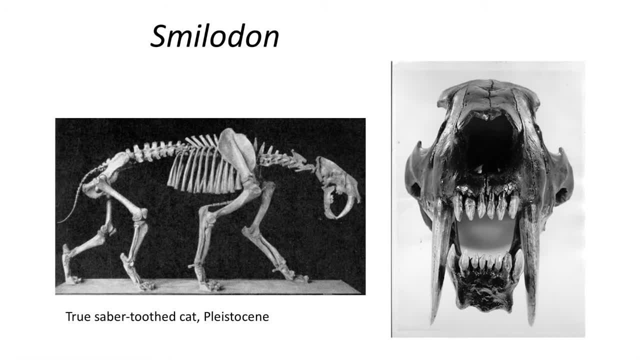 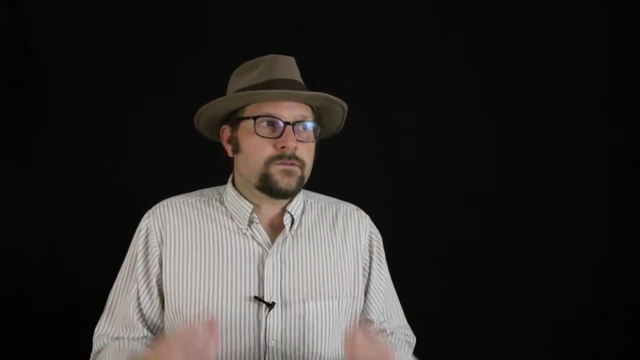 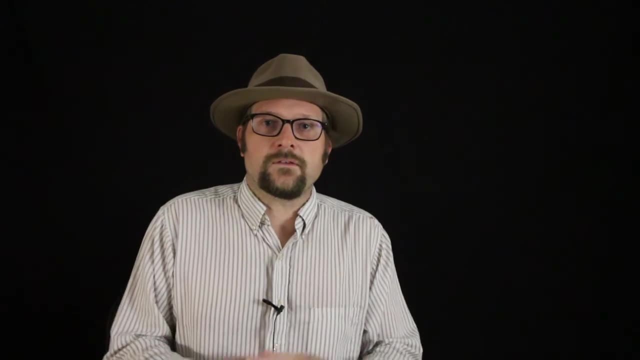 Smyrna is a female cat. Smyrna is known from hundreds of skeletons from Los Angeles, from the La Brea Tar Pits locality near Hollywood. So why did long saber-toothed mammals appear to evolve multiple times? One theory is that these long saber teeth were an effective tool for subduing larger 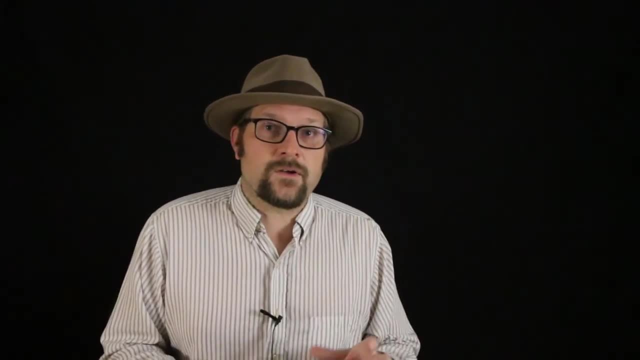 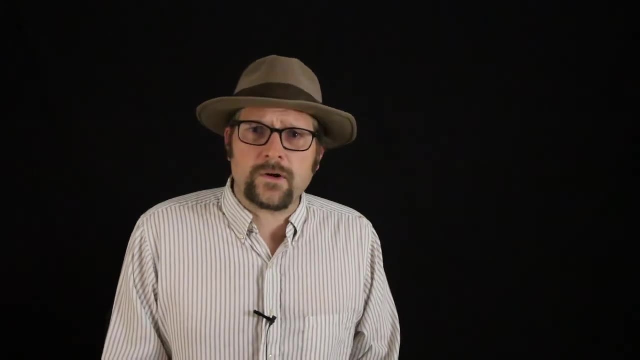 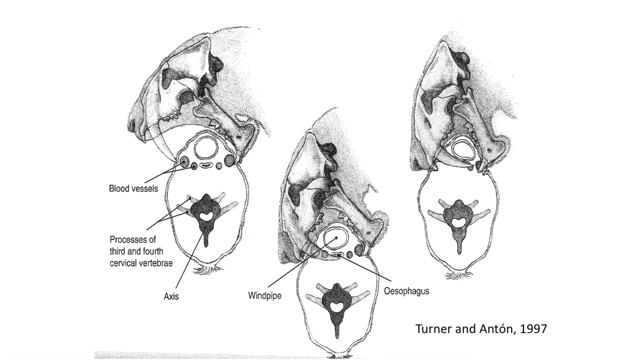 prey, Like when a big cat tries to take down a larger hoofed mammal, it risks getting kicked in the mouth or stabbed with nasty horns. So the cat goes after the vital organs in the throat, including the carotid blood vessels. 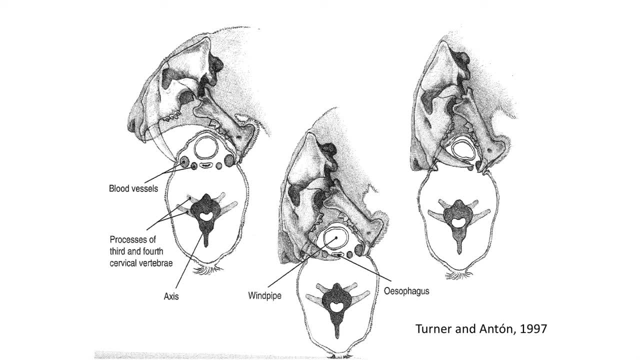 knocking out brain function as well as the trachea, which quickly disrupts airflow into the lungs. A ripping out throat is one way to knock down a larger predator and hence feed the family for a longer period of time than carnivorous animals. The long saber-toothed cat is one way to knock down a larger predator and hence feed the family for a longer period of time than carnivorous animals. The other group of oligocene to modern carnivores includes the caniforma. These include the canid family, the modern dogs, as well as a group called the arctodidae. 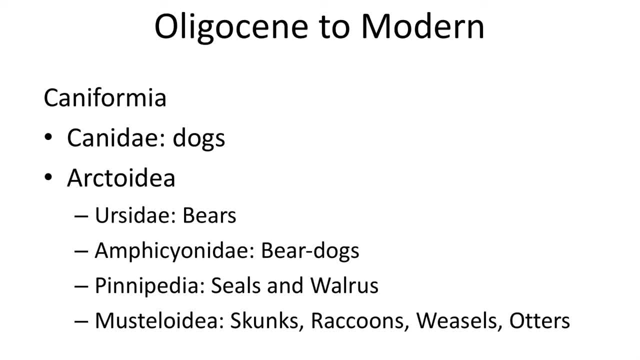 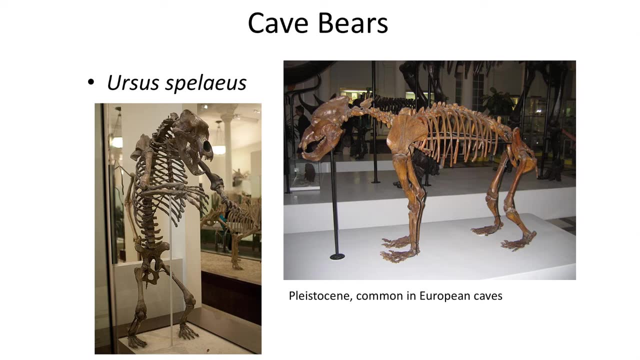 which includes bears, bear dogs, seals and walruses, as well as diverse mustelidae, the skunks, raccoons, weasels and otters, And fossils from this group are impressive. Ancient cave bears are found across Europe from the late Pleistocene, living alongside 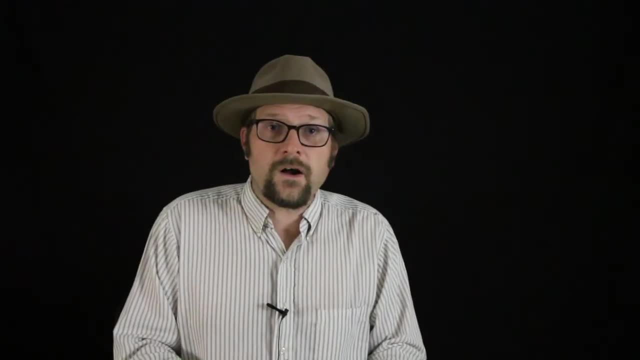 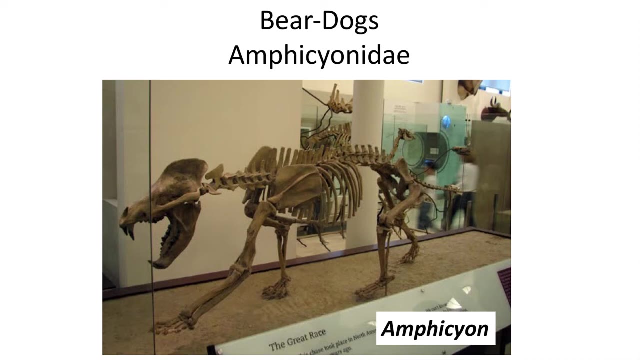 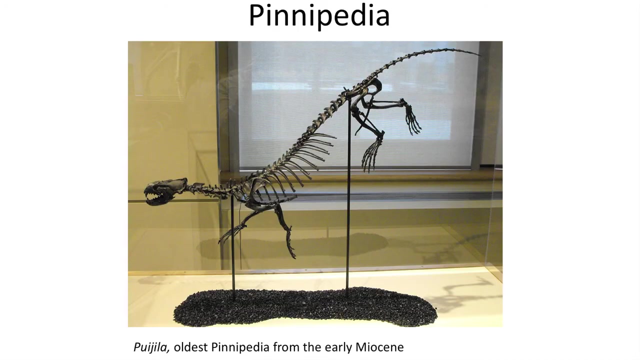 humans in Europe during the Ice Age. Bear dogs lived during the Miocene and were large, ground-adapted bear-like mammals with massive skulls. Pinnipedae, the group that would evolve into seals and walruses, have a fossil record extending. 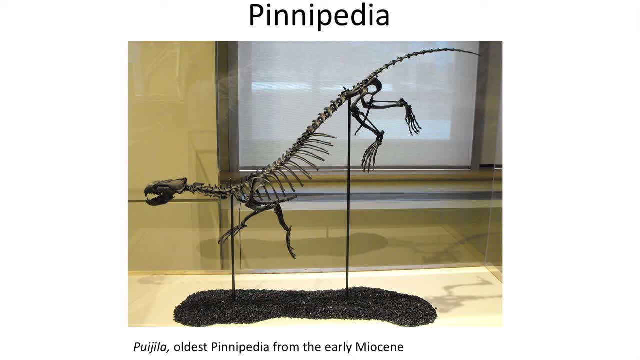 into the early Miocene Pinnipedae. the group that would evolve into seals and walruses have a fossil record extending into the early Miocene Pinnipedae. the group that would evolve into seals and walruses have a fossil record extending. 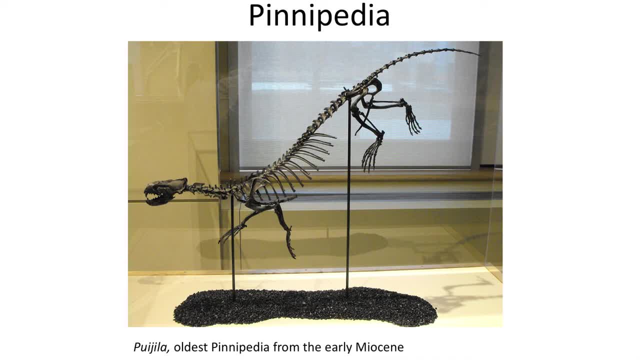 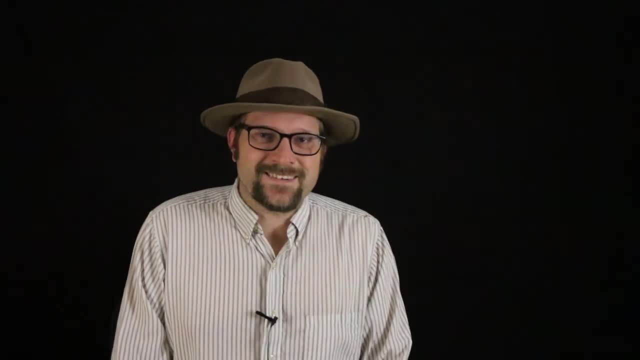 into the early Miocene. Pinnipedae, the group that would evolve into seals and walruses, have a fossil record extending into the early Miocene. These are the most famous group of mammals to make the shift into the marine environment as fully aquatic mammals, although they spend many hours on the coastlines. Alright, so we've covered a lot of groups, so let's look at how long these meat eating mammals lived by looking at their stratigraphic record. The Mesonicidae lived during the Palaeocene and Eocene. The Credonts are really two groups.